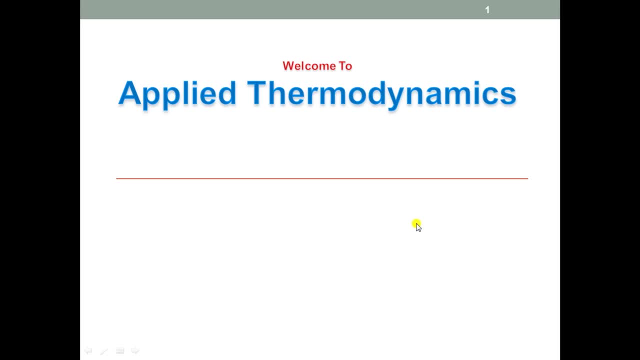 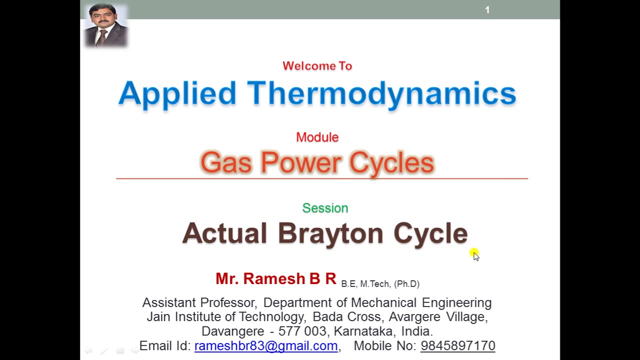 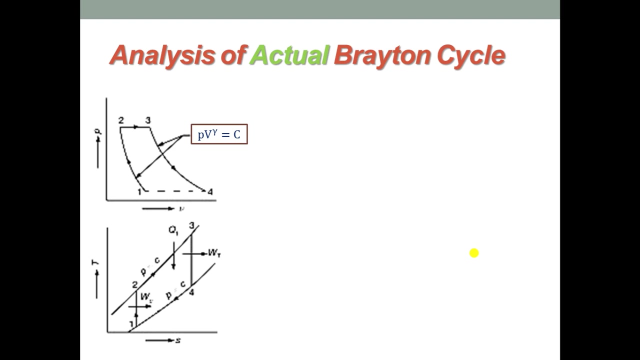 Welcome to e-learning course on applied thermodynamics, module- gas power cycles- session- actual Breton cycle. Myself, Ramesh Bir, Assistant Professor in the Department of Mechanical Engineering, Jain Institute of Technology, Downing. In this session we are going to analyze a actual 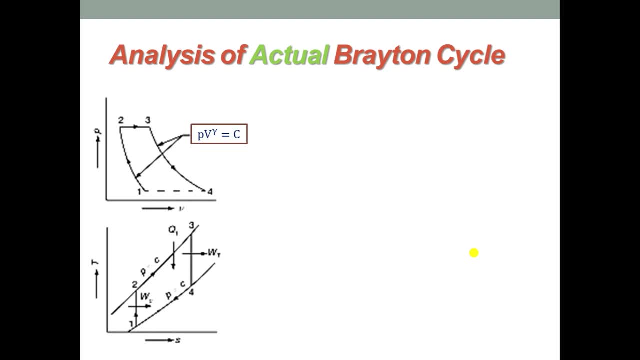 Breton cycle. The actual gas turbine cycle is different from the ideal Breton cycle due to the irreversibilities listed. The first is friction in compressor and turbine. The second one is increased gas flow through the combustion chamber and the turbine due to additional mass of fuel. 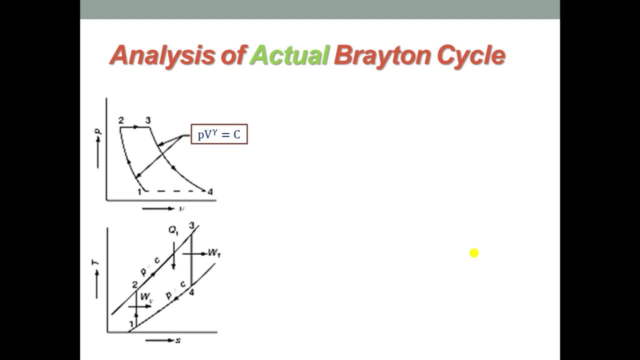 In the combustion chamber. changes in specific heat of gases and pressure drop in the combustion chamber. So these are the some of the listings based on which an actual gas turbine cycle is different from ideal Breton cycle. The irreversibilities in an actual compressor. 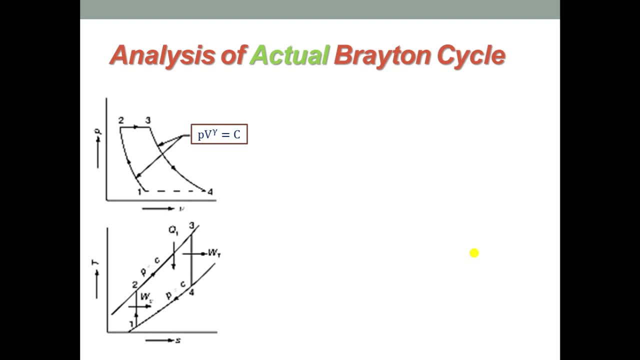 and turbine can be considered by using the adiabatic Efficiencies of the compressor and turbine as shown in the figure. The actual gas turbine cycle shown in figure with 0.1,, 2 dash, 3, 4 dash and 1.. The compressor efficiency is: 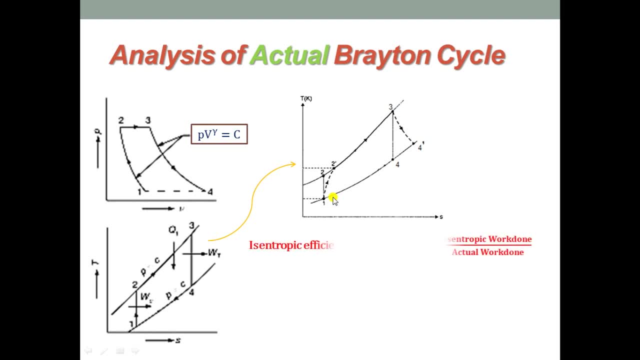 considered here, which is known as Isentropic efficiency of compressor, defined as isentropic work done by actual work done of the compressor. Based on the T s diagram, we can write isentropic efficiency as T 2 minus T 1, which is the isentropic work done during the ideal Breton cycle from 0.1 to. 0.2 over actual work done which is taken. So, based on the diagram, we can write T 2 minus T 1, to be equal to T 2 minus T 2, dash, 3, dash and 1.. Next we will discuss isentropic. 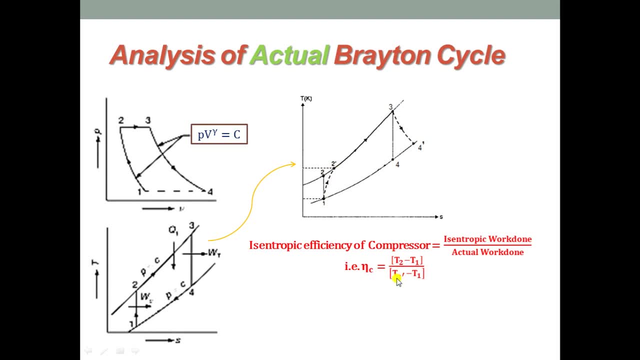 work done by actual work done by compressor. In the actual Breton cycle we can write: T: 2 is taken from 0.122 dash as T2 dash minus T1. So the ratio of these two will give the isentropic efficiency of the compression process or compressor. 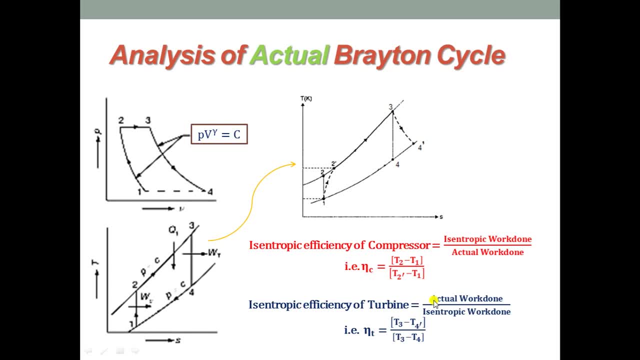 Turbine efficiency is defined as the actual work done by the turbine to the isentropic work done by the turbine. So actual work done is from 0.3 to 0.4 dash, which is taken as T3 minus T4 dash, and isentropic work done means it is ideal work done from 0.3 to 0.4. 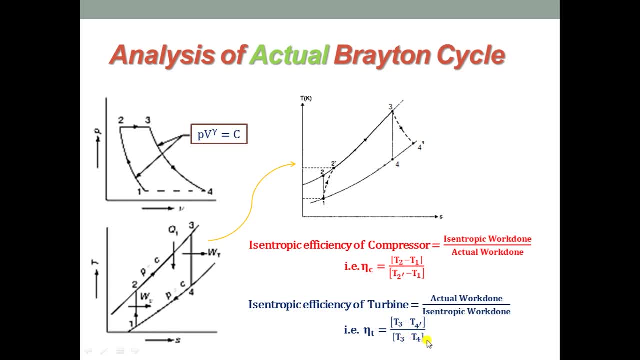 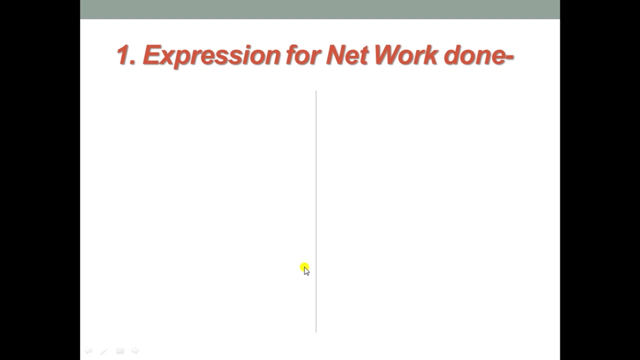 and it is taken as T3 minus T4.. So thus from these two equations it is clear that in an actual gas turbine The compressor consumes more work and the turbine produces less work than that of ideal Breton cycle. Now we see what are the expressions for net work done if it is an actual Breton. 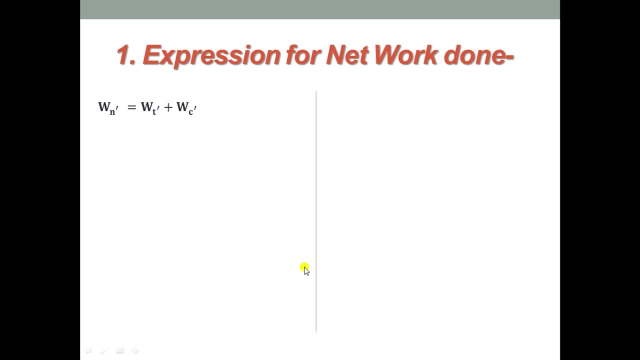 cycle. So net work done, for actual case, is given as the work done, dash, or you can also call it as prime. So work done, prime is equal to work done of turbine plus work done of the compressor, for actual case, and it is represented. 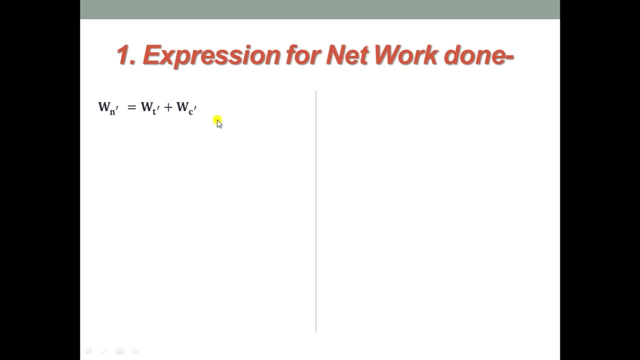 by prime to differentiate between ideal case and the actual case. So you can go through these expressions provided in the ah session: ideal Breton cycle. So this is the ideal on cycle and you can compare these 2 expressions. The work done for actual cycle based on the. 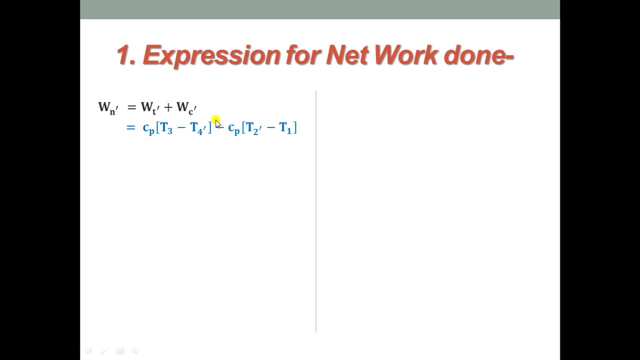 previous slide. we can refer that Ts diagram. So from there we can write the work done as Cp into T3 minus T4 prime minus Cp into T2 prime minus T1. and these 2 expressions are based on actual work done by the cycle and here negative sign represents the work done. 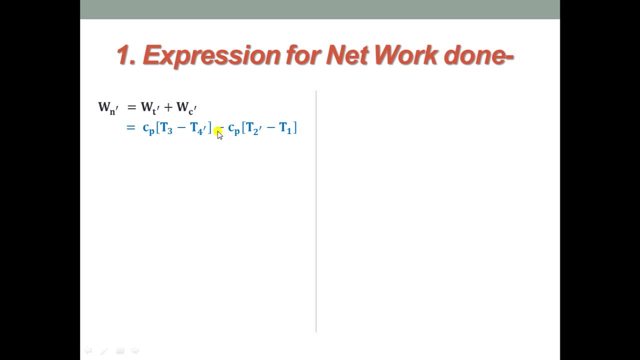 on the system by the compressor. Now we are going to use 2 very important expressions, that is, isentropic compressor efficiency and isentropic turbine efficiency, and we are going to replace T3 minus T4 prime with efficiency of the turbine multiplied with T3 minus T4 and T2 prime minus T1 with T2 minus T1 over. 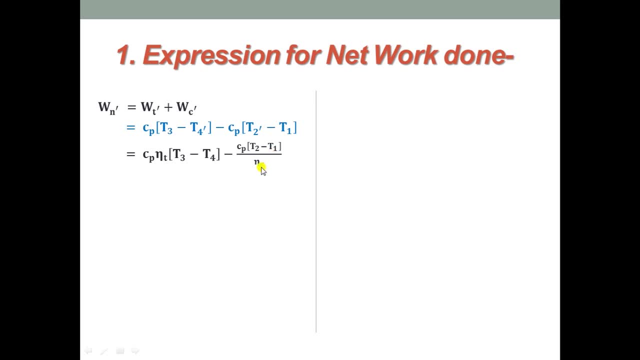 efficiency of the compressor. So these 2 expressions, how it has been replaced and what is the relation. all these things can be seen from the previous slide. Further moving with, we are going to take out maximum temperature and minimum temperature as common in these 2 terms. 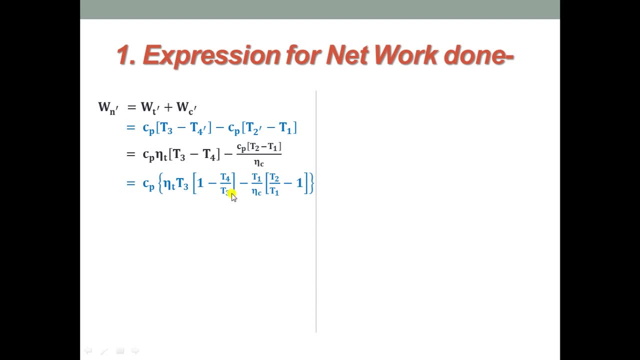 So after that we will get 1 minus T4, minus over T3, and here we will get T2 over T1 minus 1, after taking T3 and T1 as common, and Cp is common in both the terms and it is taken outside and kept in the outside the flower bracket. Hence we have the relation for T2. 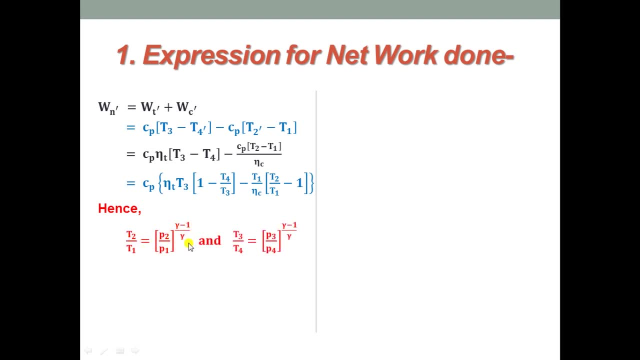 over T1, which is equal to P2 over P1 whole, to the power of gamma minus 1 over gamma, and T3 over T4 is equal to P3 over P4 whole, to the power of gamma minus 1 over gamma. So, 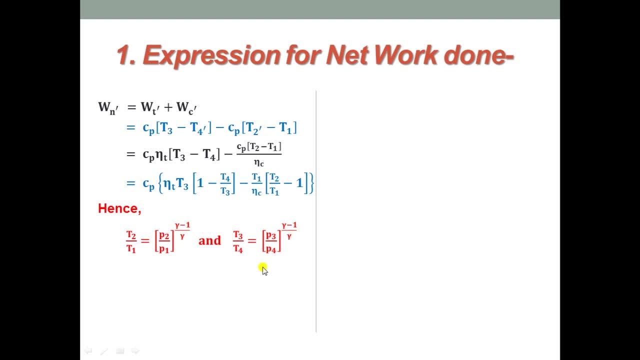 P4 whole to the power of gamma minus 1 over gamma. and these are the relations, what we will get from the process 1, 2 and 3, 4.. And then we have from PV diagram: pressure remains constant as that P2 is equal to P3 and P4 is equal to P1.. So we can say that these 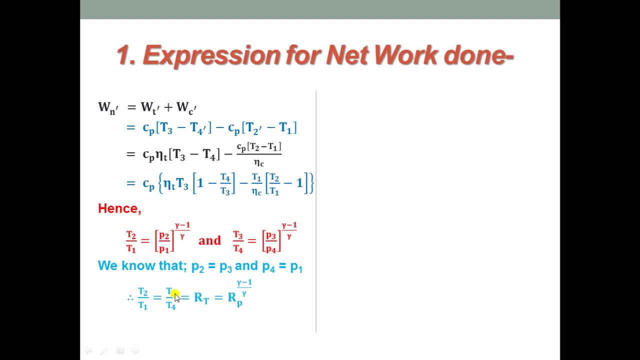 2 relations are same, So we can write it as: T2 over T1 is equal to T3 over T4, and which is taken as temperature ratio, RT, and which is also equal to pressure ratio, with power gamma minus 1 over gamma. Now we are going to replace this T4 over T3 with this relation. 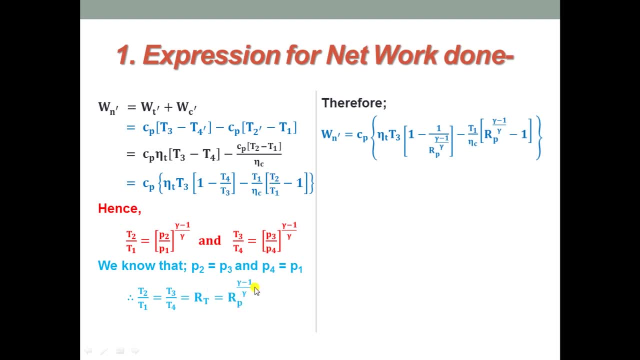 and T2 over T1. with this relation that is based on RP And after replacing the temperature ratios term with pressure ratios, we will get this expression. So now we are going to take out RP, gamma minus 1- over gamma as common in this case. So if we take common, we will. 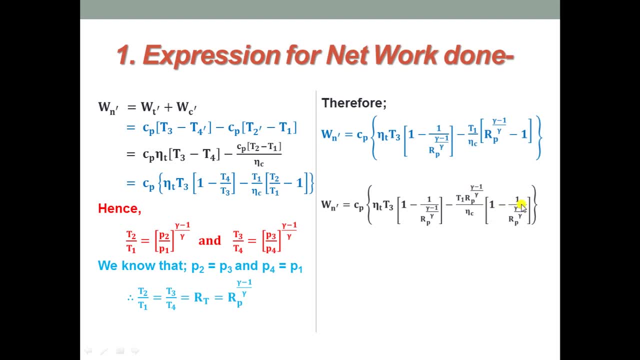 get this expression. So this is one minus 1 over RP to the power of gamma minus 1 over gamma. So now in this expression, that is, which is inside the bracket, we have common term 1 minus 1 over RP to the. 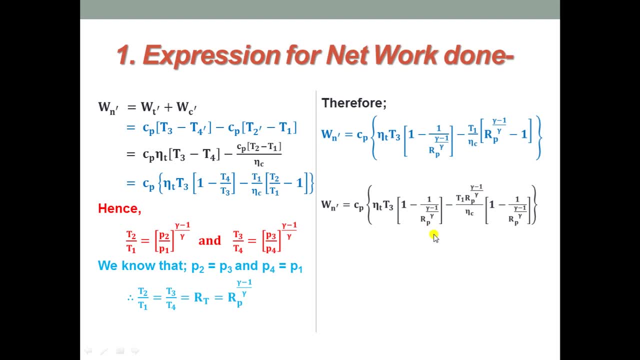 power of gamma minus 1 over gamma and it is taken outside. So as we take outside we will get this expression And the final expression for network done, for actual Breton cycle is given by C p into 1 minus 1 over RP to the power of gamma minus 1 over gamma multiplied. 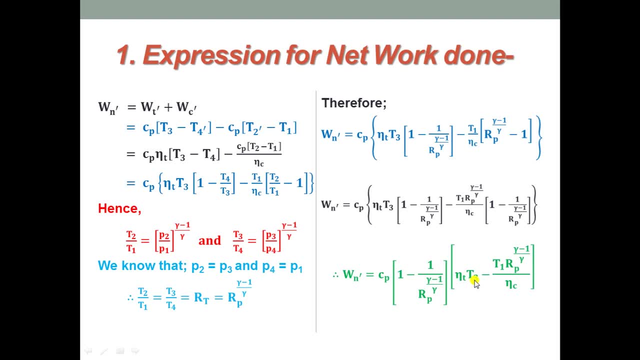 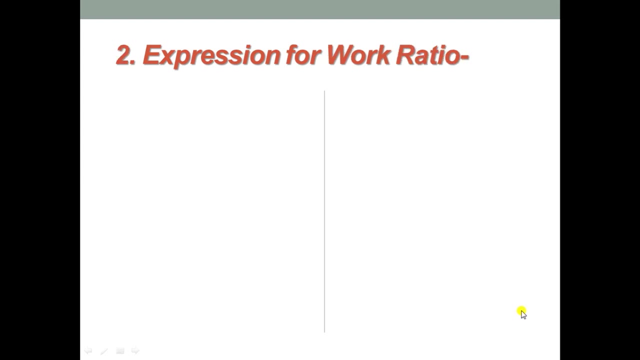 with F? u beta efficiency of the turbine multiplied with T 3 minus T 1 r p to the power of gamma minus 1 over gamma, over efficiency of the compressor. and this is the expression for actual Breton cycle. Moving on to next one, that is expression for work ratio for actual Breton cycle. So work, 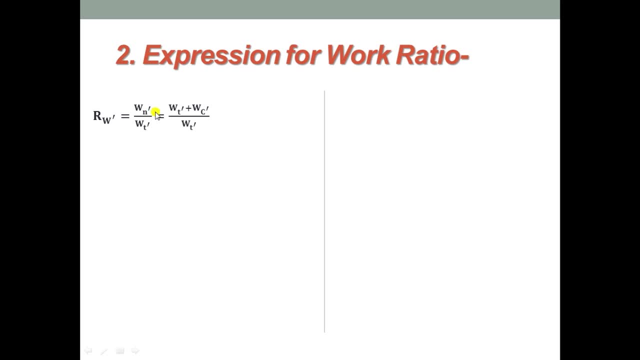 ratio is defined as the ratio of net work done to positive work and it is written as net work done. W n over positive work is turbine work. So net work done can be written as turbine work plus compressor work. Here the prime represents for actual Breton cycle and 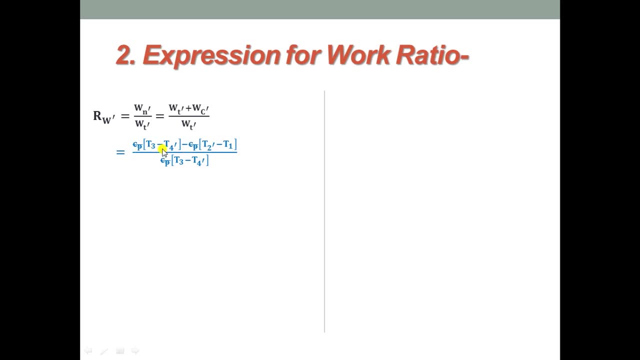 we will substitute expressions for work done: C p into T 3 minus T 4 and C p into T 2 minus T 1. over C p into T 3 minus T 4, and here negative sign represents the work done By the compressor on the system. and now we are going to cancel C p term, which is same 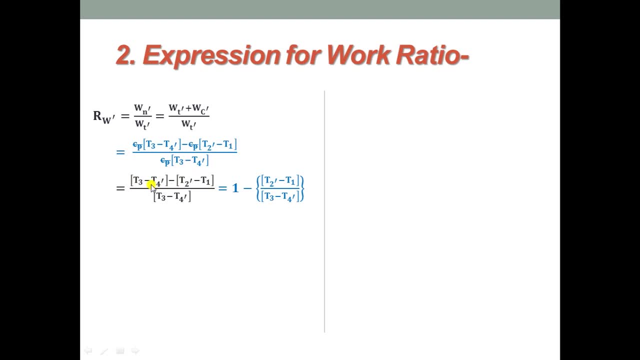 in all the 3 terms. So we will get this expression. So we are going to split numerator term into 2 part and after simplification we will get 1 minus T 2 minus T 1 over T 3 minus T 4 and 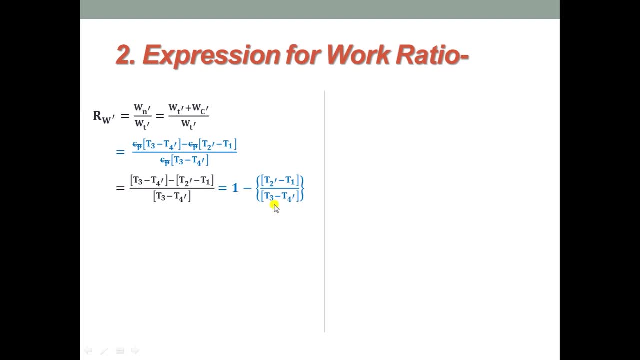 this is written for actual ideal, sorry, actual Breton cycle, And we are going to replace actual cycle with ideal cycle, considering the efficiencies of the compressor and the turbine. So we will get 1 minus T 2 minus T 1 over efficiency of the compressor over 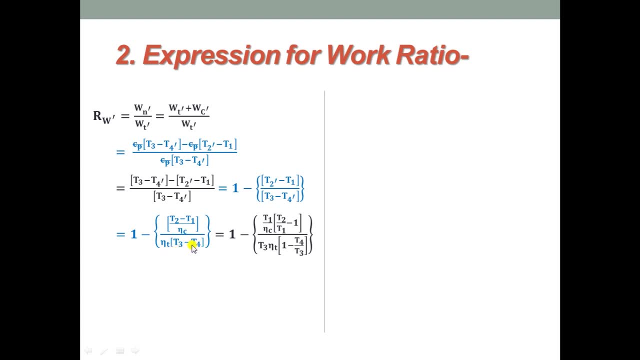 efficiency of the turbine multiplied with T 3 minus T 4.. Now in this expression we will take minimum temperature and maximum temperature as common. So that is the thing what we had made here and here. So hence we have the relation T. 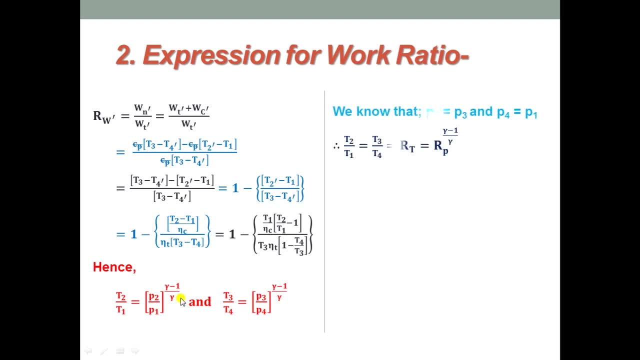 2 over T 1 and T 3 over T 4, based on the pressure ratios. And we know that P 2 is equal to P 3 and P 4 is equal to P 1.. So from your P V diagram and the expression for pressure, 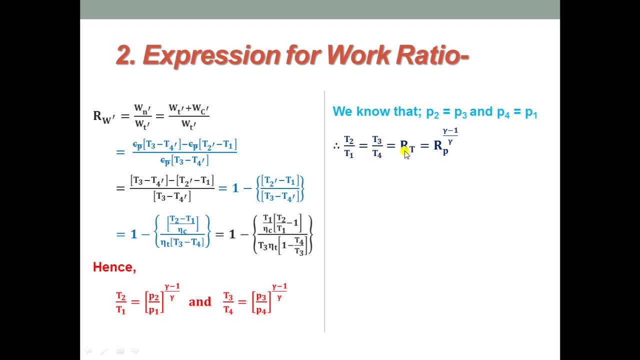 ratio and temperature ratio can be written as: T 2 over T 1 is equal to T 3 over T 4, which is equal to temperature ratio, and pressure ratio over gamma is 1 over gamma, And we are going to replace T 2 by T 1 and T 4 by T 3 as temperature ratio, R, T And this is the 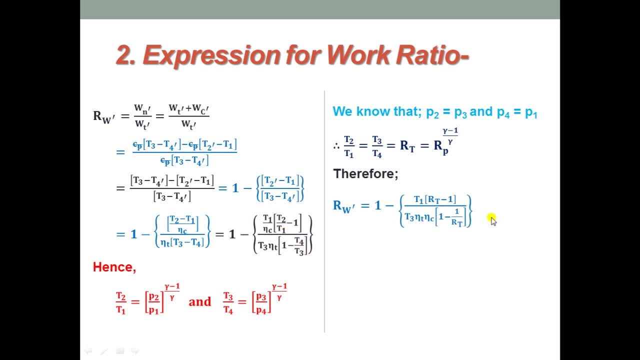 expression what we will get after replacing T 2 by T 3.. Question Time: Professionals- Professionals: Professionals: 2 over T 1 and T 4 over T 3, and now we are going to take out R T as common here and this. 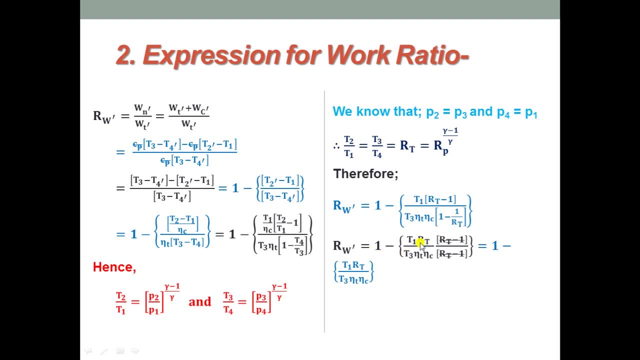 is the expression, what we will get, and then this becomes: 1 minus T, 1. R T over T 3: efficiency of the turbine into compressor turbine. here This is the expression what we will get after cancelling R T minus 1 term, and the final expression becomes: by replacing R T with R. 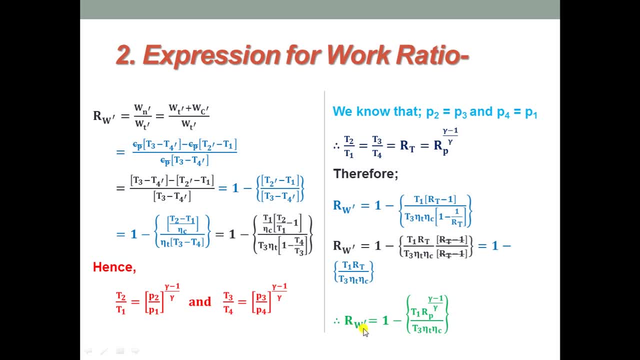 P gamma minus 1 over gamma and the work expression or work ratio expression for actual Brayton cycle is given by 1 minus T 1 R P gamma minus 1 over gamma over T 3 into turbine efficiency and compressor efficiency. and this is the expression for work ratio of actual Brayton. 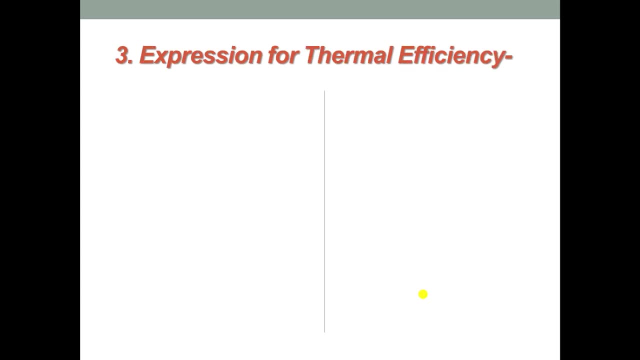 cycle. So moving on to next one, that is thermal efficiency of the actual Brayton cycle. So it is defined as net work done by heat added. So net work done can be written as turbine work plus compressor work. So turbine work is given by C p into T 3 minus T 4 for actual 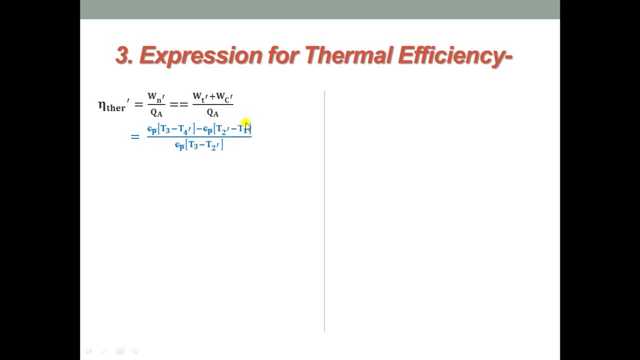 case and C p into T 2 minus T 1 for actual case of compressor, and negative sign represent work done on the system and heat added is given by C p into T 3 minus T 2.. So C? p get cancelled and the final expression becomes like this: 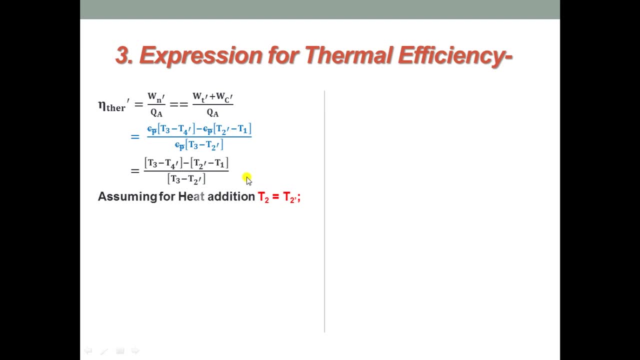 Now, in this we are going to interchange the temperature terms. So, as we know that we are going to make some assumption here before going to interchange the temperature term, that is So T 2 dash or T 2 prime is equal to T 2, we are going to consider that assumption. 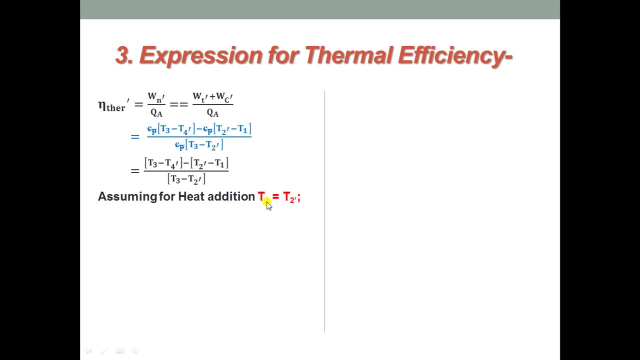 for heat addition, that is, initial temperature of the heat addition process. So for that. so after making this, we are going to replace T 3 minus T 4 prime as efficiency of the turbine to T 3 minus T 4.. And T 2 prime minus T 3 minus T 4 prime is equal to T 3 minus T 4.. 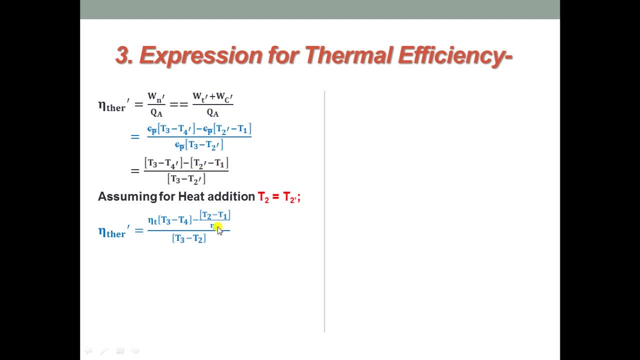 So T 1 is equal to T 2 minus T 3 minus T 4, T 1 as T 2 minus T 1 over efficiency of the compressor. and here we are going to make out in the denominator part with T 1 that 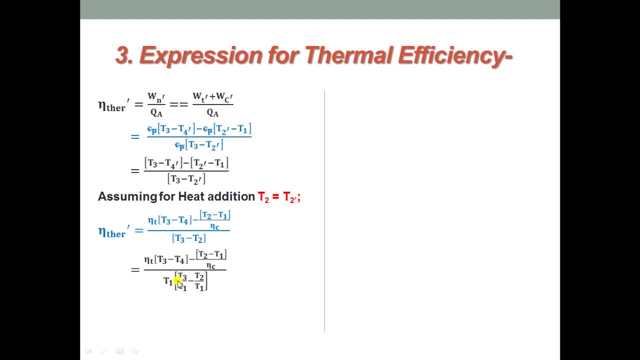 is, we are going to multiply and divide with T 1 in the denominator part. So then we are going to get this expression by taking T 3 as common in the first term and T 1 as common in the second term. we have the relation for T 2 over T 1 and T 3 over T 4, as well as we know that P 2 is. 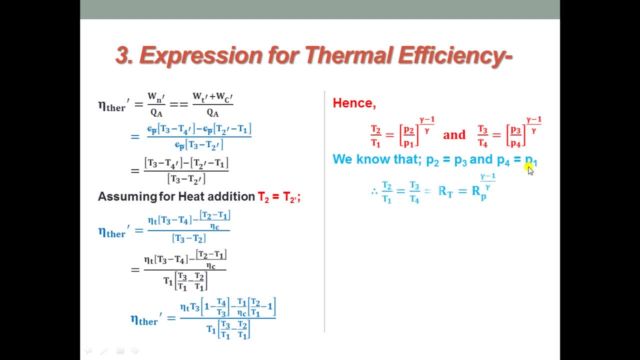 equal to P 3 and P 4 is equal to P 1.. So, and the final relation, what we will get is T 2 over T 1 is equal to T 3 over T 4, which is equal to R T. that is temperature ratio. 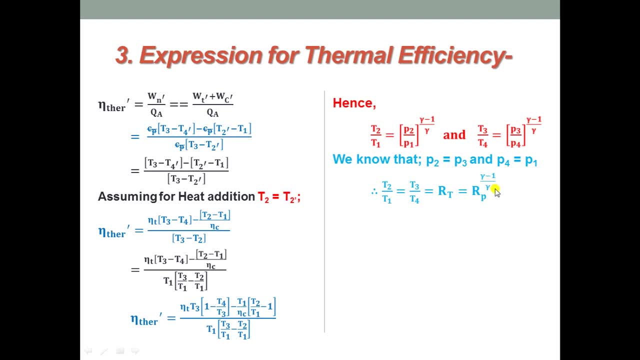 which is also equal to pressure ratio, with the power gamma minus 1 over gamma. Now we are going to replace the ratios with T 4 over T 3 and T 2 over T 1 and T 2 over T 1 with R P value. that is pressure ratio And the final expression is given by: for thermal: 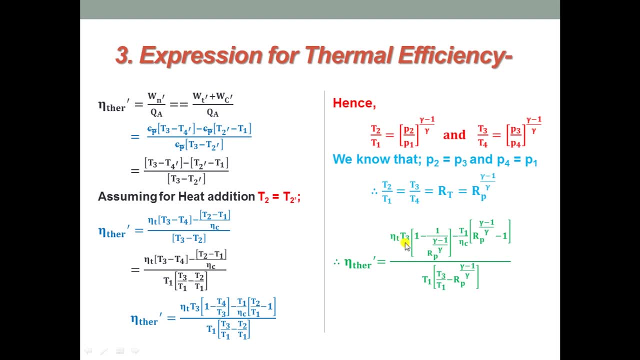 efficiency of actual Brayton cycle as efficiency of the turbine multiplied with T 3, multiplied with 1 minus 1 over R P, to the power of gamma minus 1 over gamma minus T 1 over efficiency of the compressor multiplied with T 2 over T 3.. 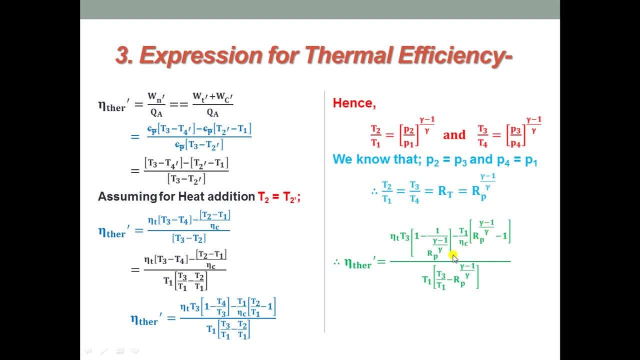 So with R P to the power of gamma minus 1 over gamma minus 1 over T 1, T 3 over T 1 minus R P to the power of gamma minus 1 over gamma, And this is the expression which is used to. 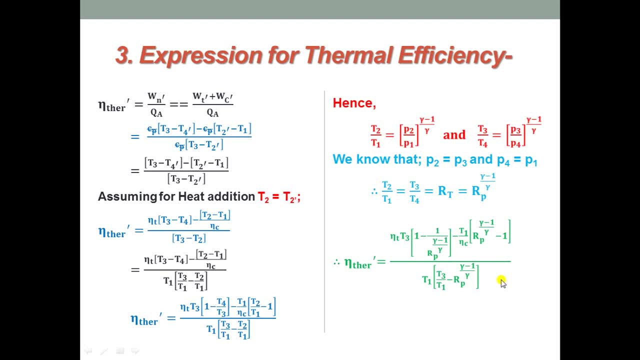 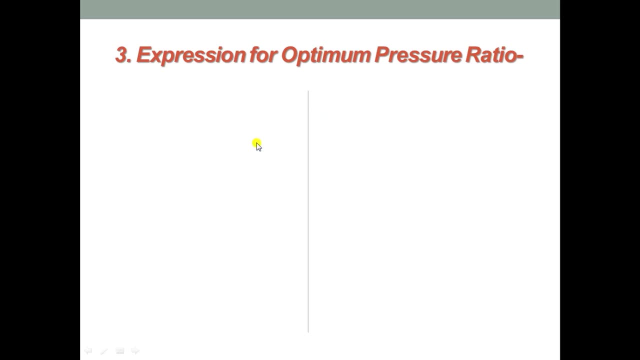 obtain thermal efficiency of the actual Brayton cycle, Moving on to the last one, that is, optimum pressure ratio. So as we know, to get optimum pressure ratio we are going to differentiate net work done with respect to pressure ratio. So first We will write net work done expression, So that is turbine work plus compressor work. 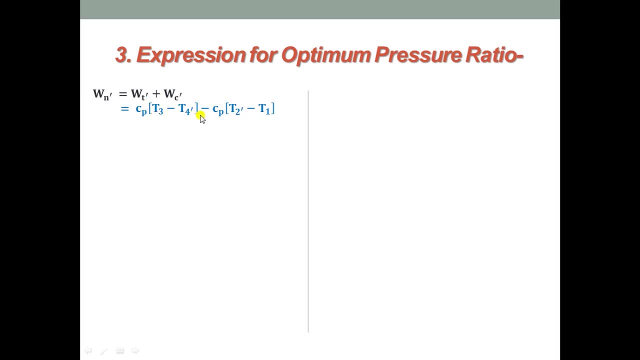 So equation for turbine is C p into T 3 minus T 4 and equation for compressor is minus C p into T 2 minus T 1, and it is written for actual Brayton cycle. Now we are going to replace actual with ideal by using turbine, efficiency and compressor. 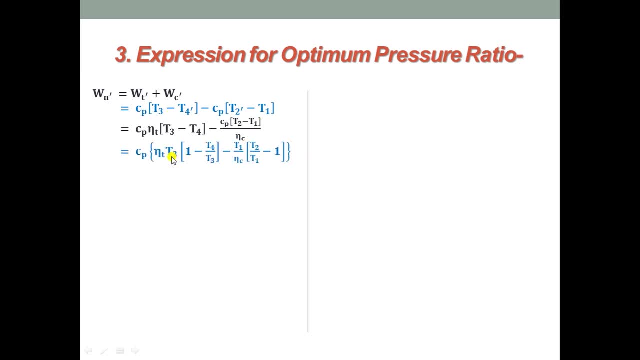 efficiency, And we are going to make out T 3 and T 1 as common here, and C? p is common in both the terms and the final expression is this: And hence we have the relation for T 2 over T 1 and T 3 over T 4, as P 2 over P 1, whole to the power of gamma minus 1 over 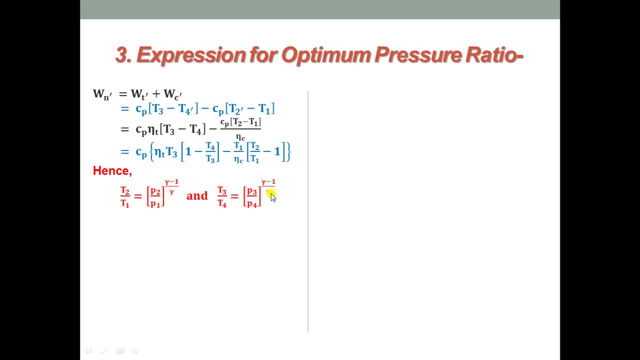 gamma and P 3 over P 4 whole to the power of gamma minus 1 over gamma. We know that P 2 is equal to P 3 and P 4 is equal to P 1 from your P V diagram, So we can write. 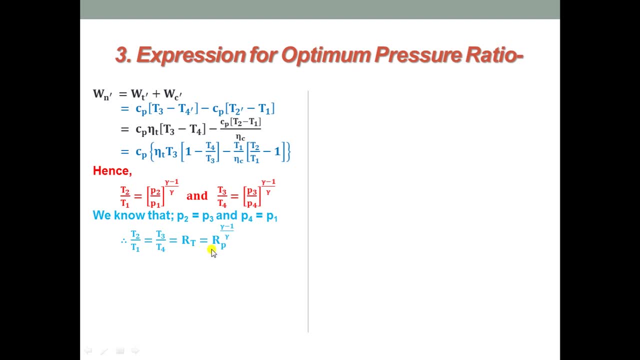 T 2 over T 1 is equal to T 3 over T 4, which is equal to temperature ratio, which is equal to pressure ratio, with power gamma minus 1 over gamma. Thank you. Now we are going to replace T 4 over T 3 and T 2 over T 1 in this expression with pressure. 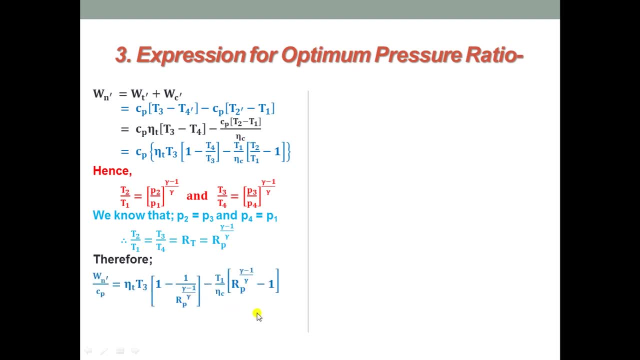 ratio or temperature ratio. So we have replaced with pressure ratio and C. p is taken on to the left side and it becomes denominator below network done. And to simplify the complexity of this expression, we are going to take gamma minus 1 over. gamma is equal to m and we are 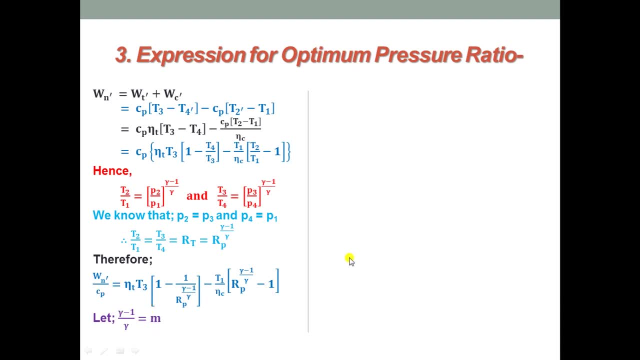 going to replace this in this expression. After that, we are going to replace this in this expression. So, after replacing that, so we are going to get this expression. So that is: network done by C p is equal to turbine efficiency of T 3 multiplied with 1 minus 1 over R p to the 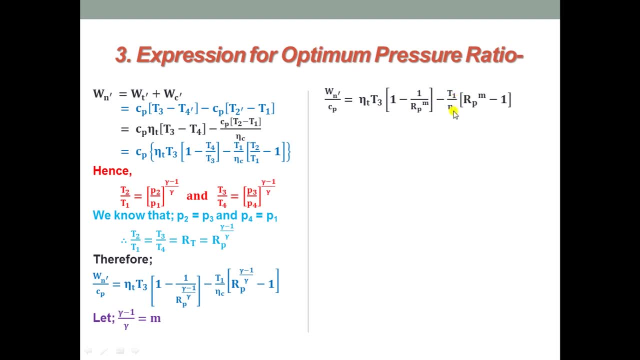 power of m minus T, 1 over efficiency of compressor multiplied with R p to the power of m minus 1.. Now we are going to differentiate this expression with respect to pressure ratio on both sides. So network done by specific heat, this compression. So we are going to 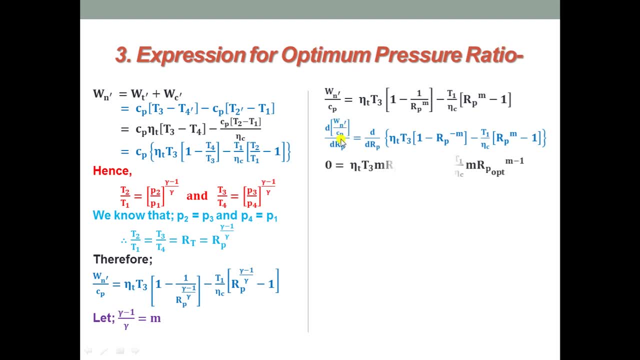 take this full� гру wane and this complete term will be constant And differentiating constant becomes 0,. differentiating the first term will get efficiency, or the turbine is a constant term. remains as it is. temperature is also constant. remains as it is. 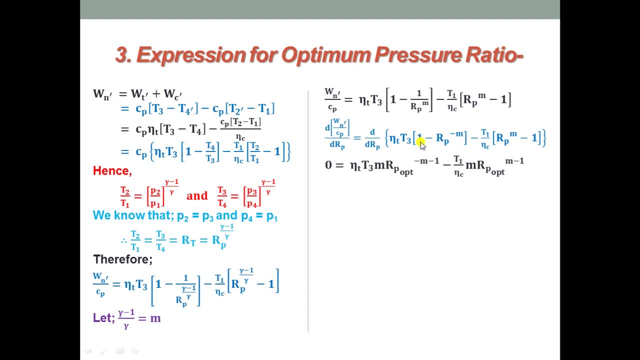 And differentiating 1 minus 1, the constant 1 is also 0. And we get positive of m R p to the optimum and the power becomes minus m minus 1.. Similarly, second term will get 1 efficiency as constant it it is taken outside and differentiating r p, m minus 1 will get. 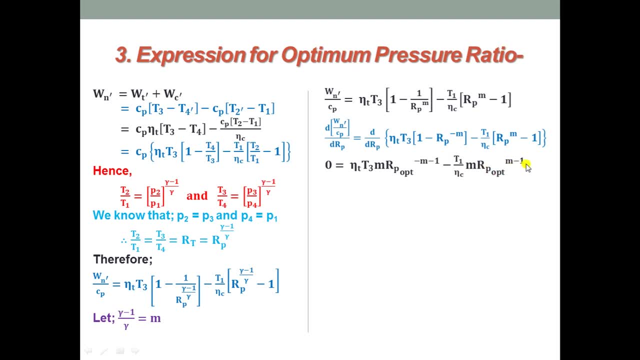 r p 2 m into r p to the optimum m minus 1.. Now we are going to replace or rearrange the terms, So, moving this negative term on to the other side, we will get positive and m get cancelled on both sides. Now we are going to write this expression in the form: 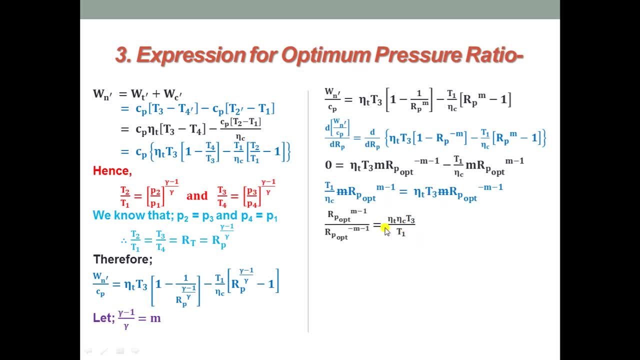 of pressure ratio as well as temperature ratios. So we will get this expression and we are going to move r p optimum into the numerator. So we will get this. So the power becomes m minus 1 plus m plus 1 and on the other side it remains as it is: turbine efficiency. 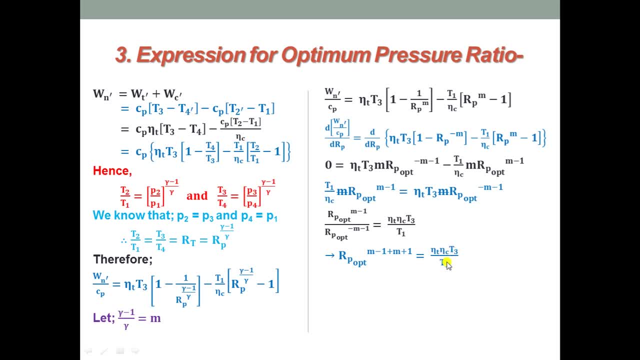 multiplied with compressor efficiency, multiplied with T 3 over T 1.. So after this, so we will simplify the power. So finally we will get R p optimum 2 m as power which is equal to efficiency of turbine efficiency of compressor, multiplied with T 3 over T 1.. Now we are going to move the power of pressure. 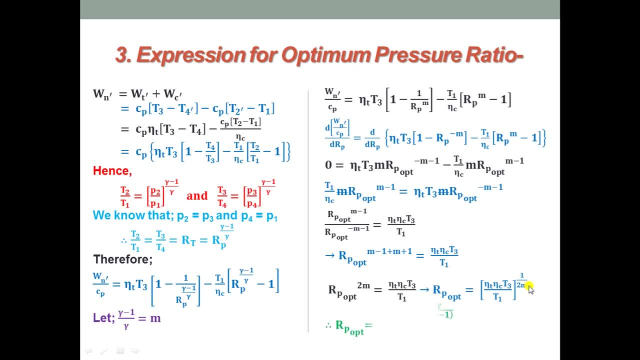 optimum on to the other side it becomes 1 over 2 m and the final expression: what we will get here by replacing m with gamma minus 1 over gamma, with m as m. So we will get R p optimum foractual cycle as efficiency of the turbine multiplied with efficiency.